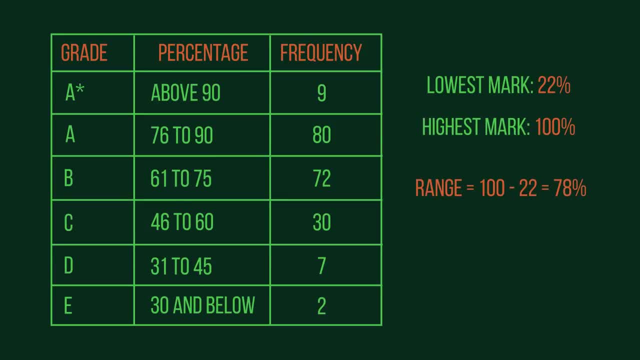 these groups is the same. Let's try and make them more equal. We know the lowest mark was 22% and the highest mark was 100%, So the range of results is 78% Now because we have A star, A, B, C, D and E, so 6 groups work out approximately how. 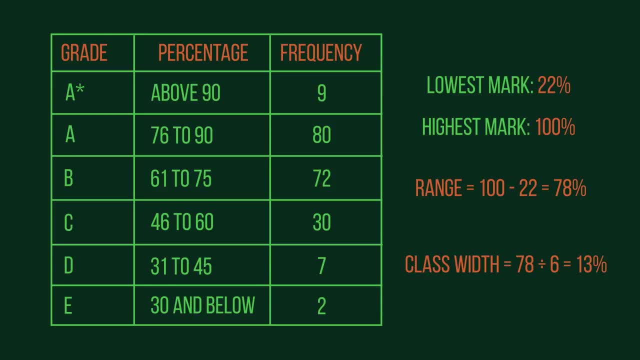 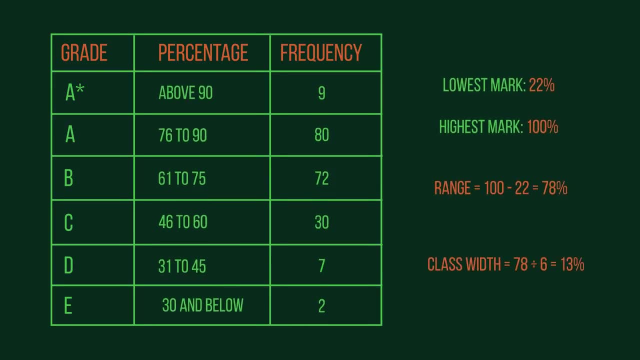 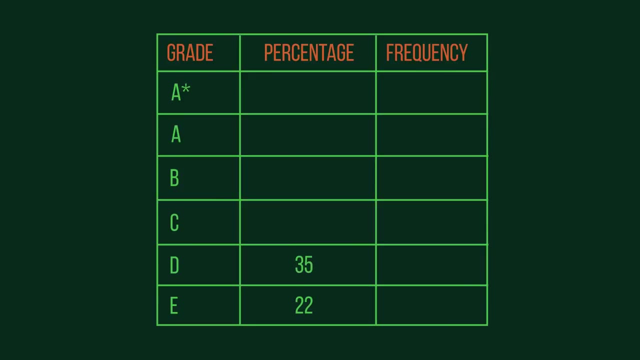 big each group should be by dividing the range by 6.. We want each group to be about 13% in size, Starting from the bottom at 22.. Add 13.. 12 plus 13 is 35. So the next group starts at 35.. 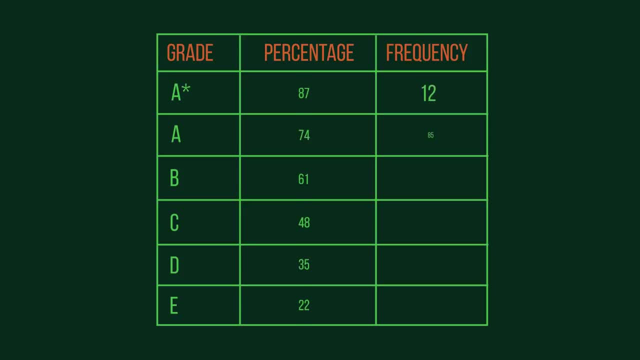 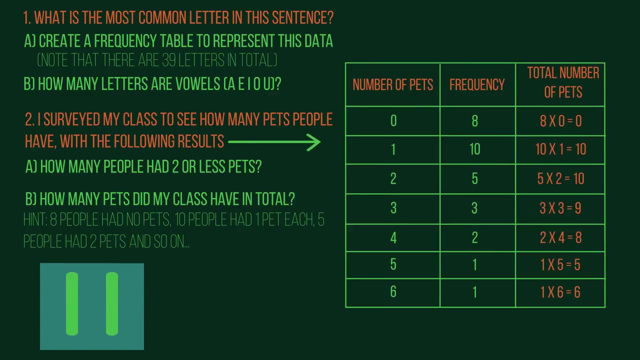 Adding 13 each time. 3. Fill in the rest of the group at the end. We now have 6 groups that are pretty much the same class width. Here are some questions for you to do. Pause the video, work them out and click play when. 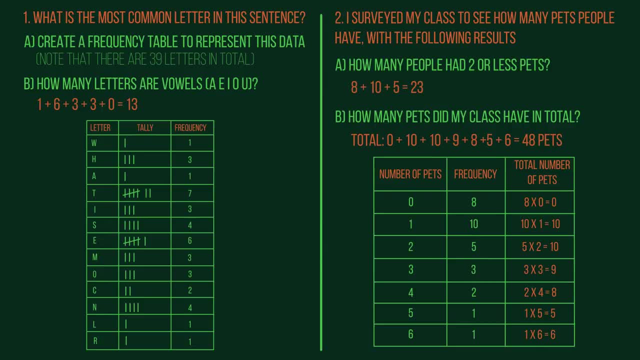 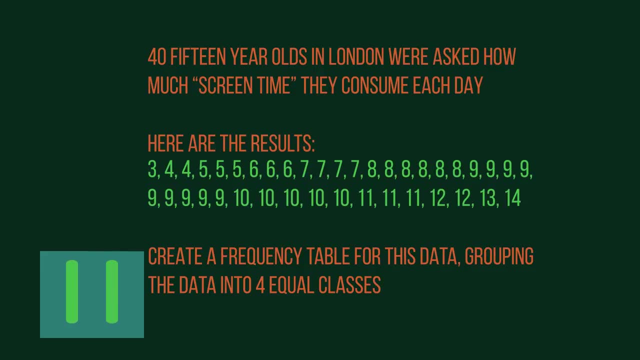 you're ready. How'd you get on? One final question for you to do: Create 4 equal groups or classes for this data. Pause the video, work it out and click play when you're ready. Did you get the groups right? 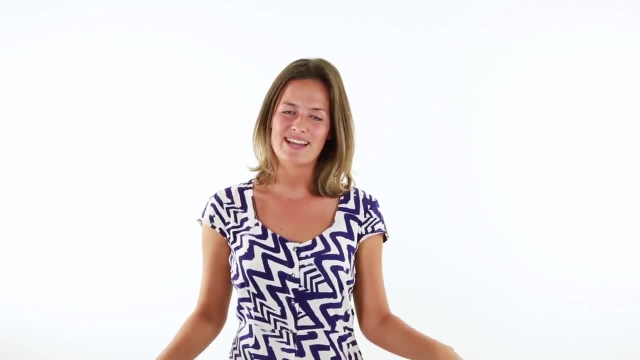 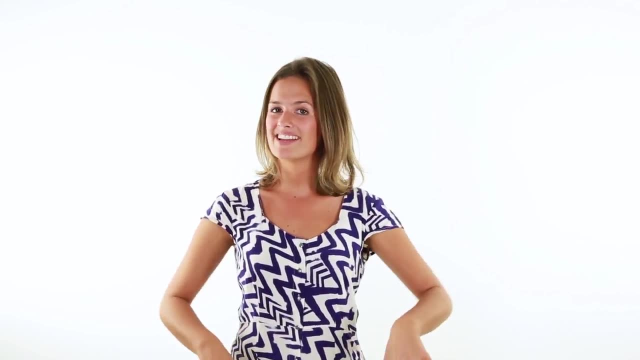 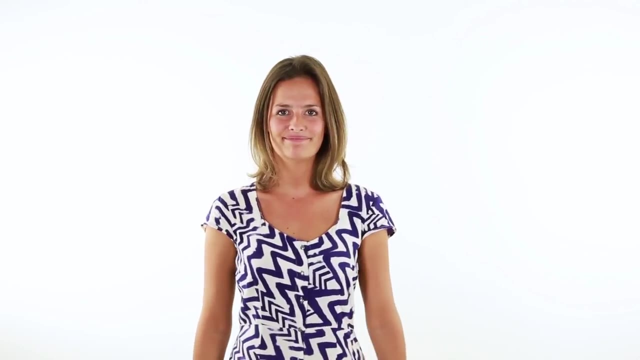 So that's the end of frequency tables. They're very useful for collecting data together to make it much easier to handle. We can then calculate averages or draw different graphs from them, like histograms, which we'll look at in another video. If you liked the video, give it a thumbs up and don't forget to subscribe. Comment below. 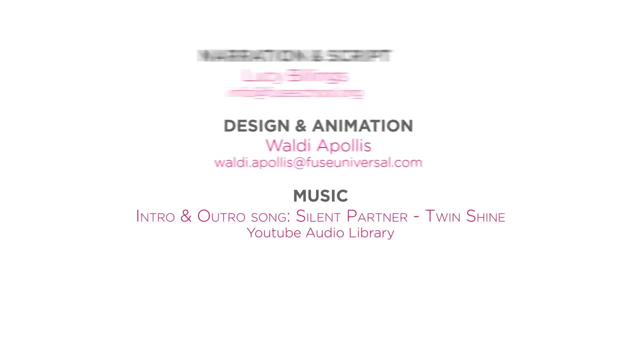 if you have any questions, Why not check out our Fuse School app as well? Until next time,